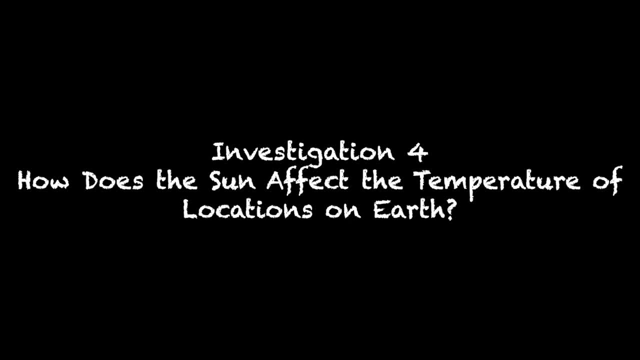 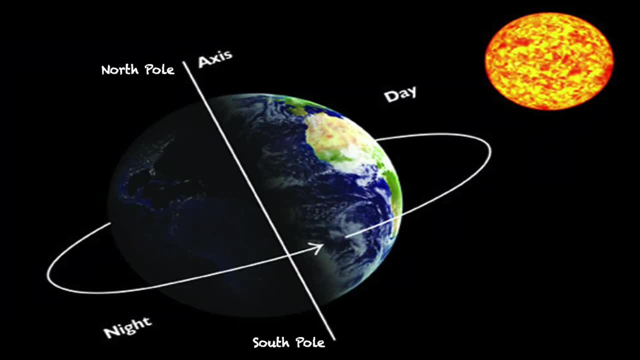 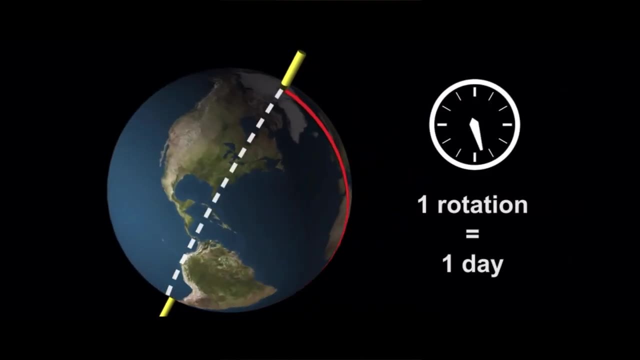 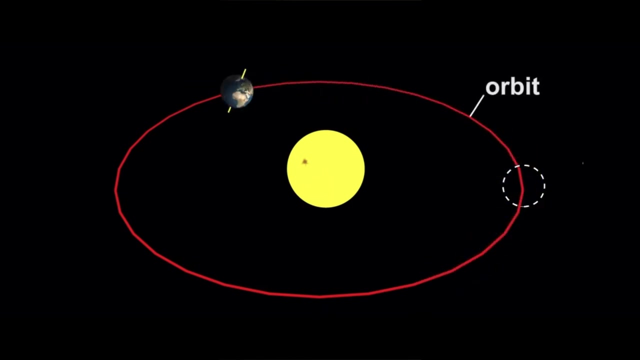 Earth turns on an imaginary line called its axis. The north and south poles are at the ends of this axis. The motion is called rotation. It takes just about 24 hours for Earth to make one rotation. Earth travels in a slightly elliptical orbit around the sun, with one revolution taking 365. 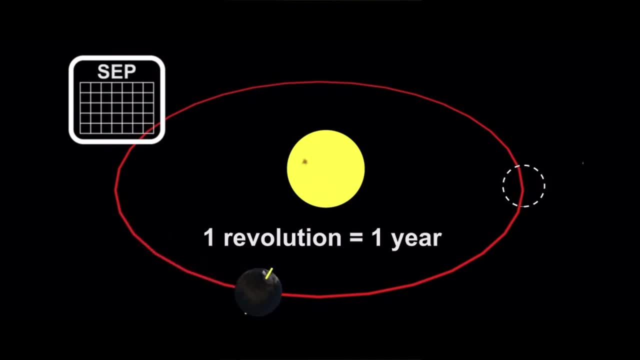 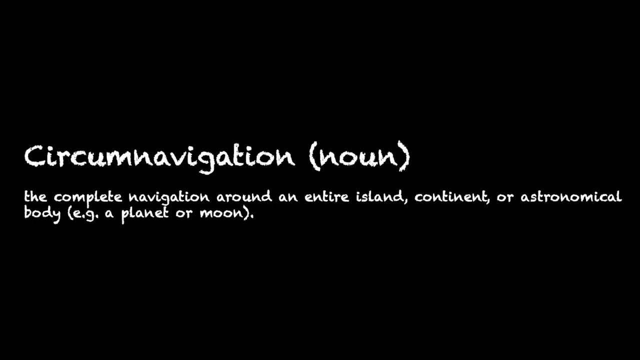 and a quarter days. The average distance between the sun and Earth is 149.6 million kilometers, but because Earth's orbit is not quite round, Earth is predictably farther from and closer to the sun during its annual circumnavigation Perihelion, which is the 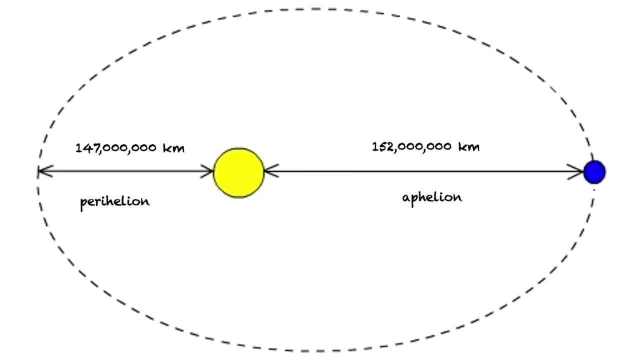 closest point occurs about January 3rd and the distance is 147 million kilometers. Aphelion, which is the closest point, occurs about January 3rd and the distance is 147 million kilometers. Perihelion, which is the furthest point, occurs about January 4th and the distance is 152 million. 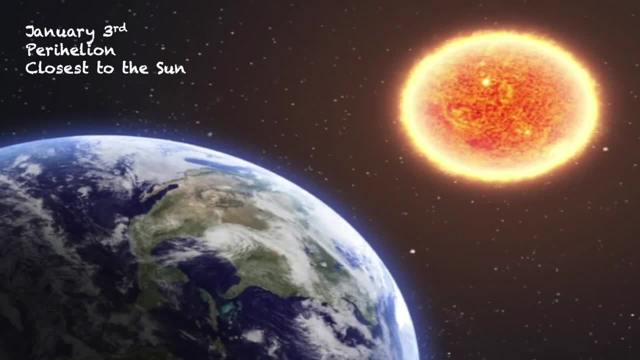 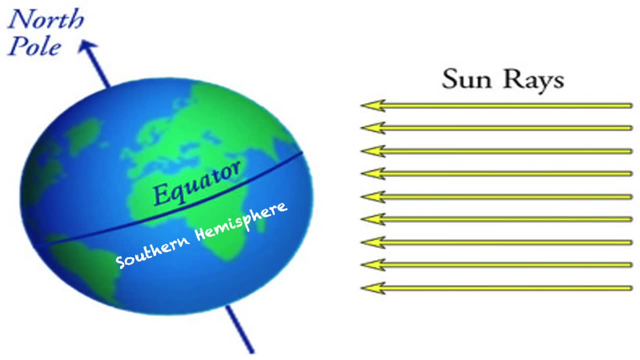 kilometers Because Earth is closest to the sun around January 3rd. common sense might suggest that is when Earth would be warmest. People in the southern hemisphere would nod in agreement because January is summer down there In the northern hemisphere. however, we know this is. 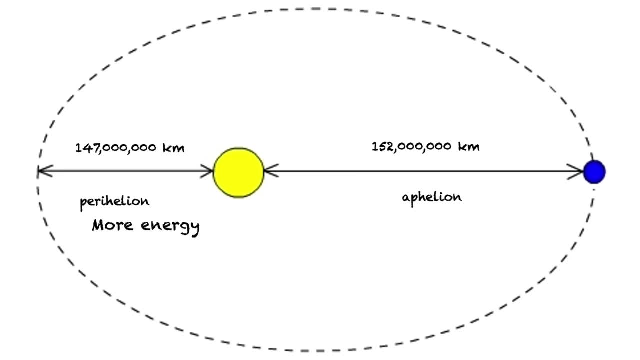 not the case. Earth as a whole does receive more energy from the sun in January at any other time of the year, but that is not the reason for the seasons. Proximity to the sun is not the variable that determines summer and winter. It's the tilt of. 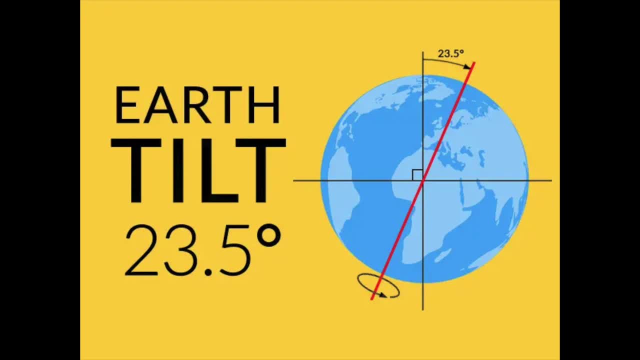 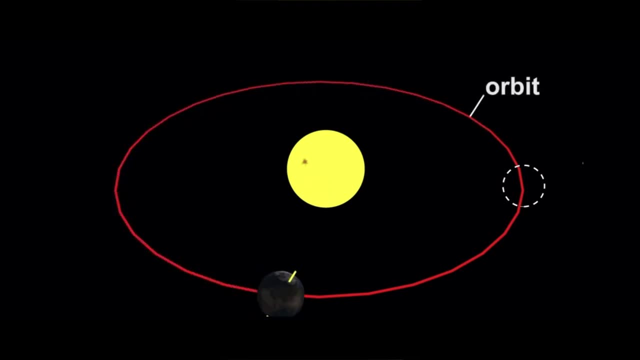 Earth's axis. Earth's axis is tipped by 23.5 degrees from vertical with respect to the plane of its orbit around the sun. As Earth revolves around the sun in its elliptical orbit, it also rotates on its tipped axis- one rotation every 24 hours. 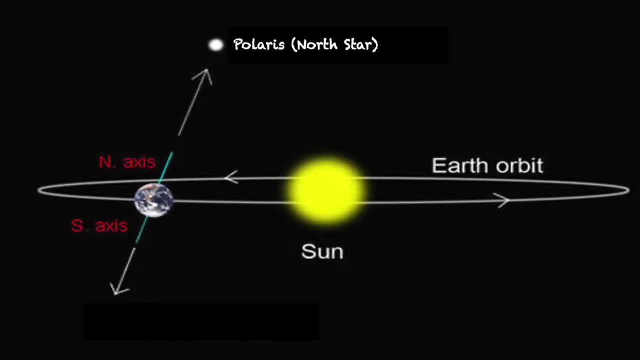 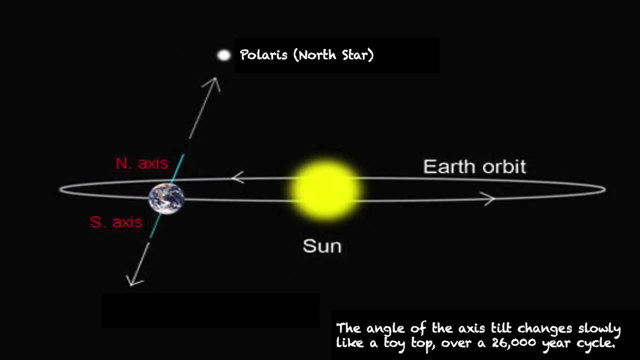 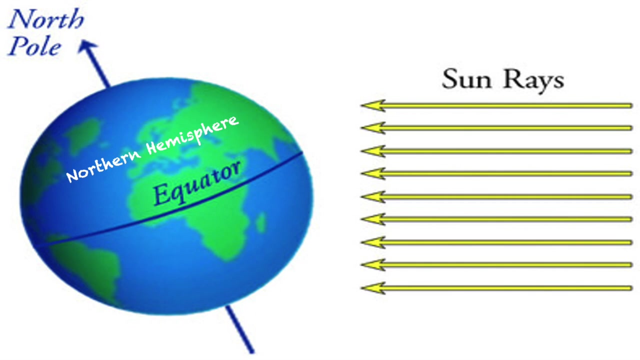 By coincidence, the North Pole aims towards a star called Polaris or the North Star. At this time in history, no matter where Earth is in its orbit, the North Pole always points towards the North Star. During Perihelion, the North Pole is leaning away from the sun. This is the time of 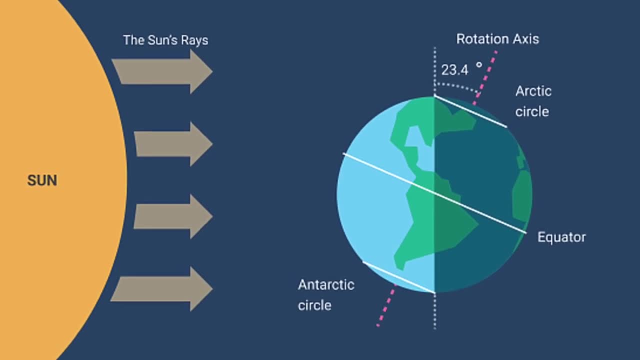 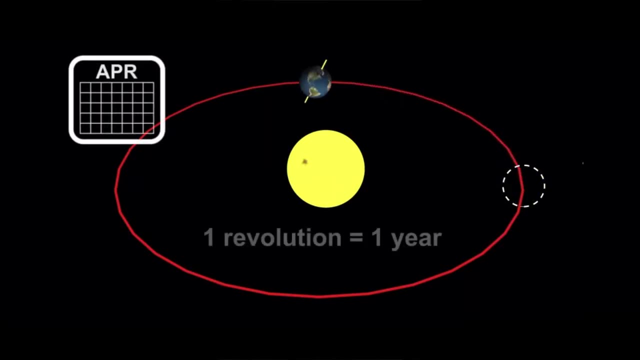 darkness. for Earthlings living north of the Arctic Circle, Days are shortest and nights are longest. for the northern hemisphere, This season is winter. Half a revolution later, the North Pole is leaning away from the sun. This is the time of darkness for Earthlings living. 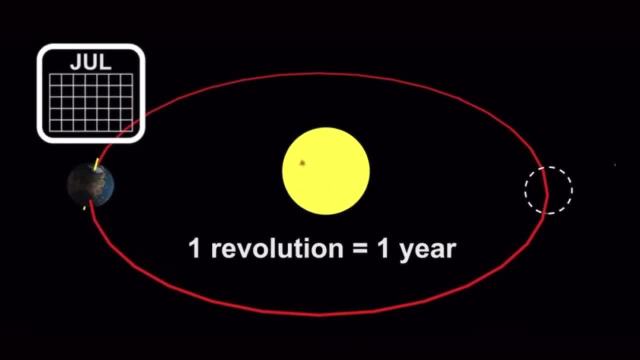 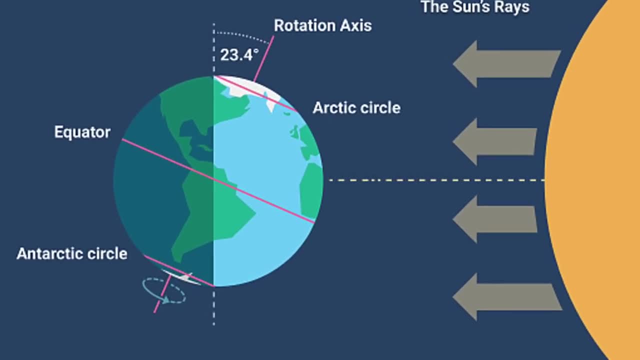 north of the Arctic Circle. The South Pole, still pointing at the North Star, is leaning towards the sun. The days in the northern hemisphere are longer. At the same time, the South Pole angles away from the sun and the southern hemisphere experiences shorter days and longer nights. 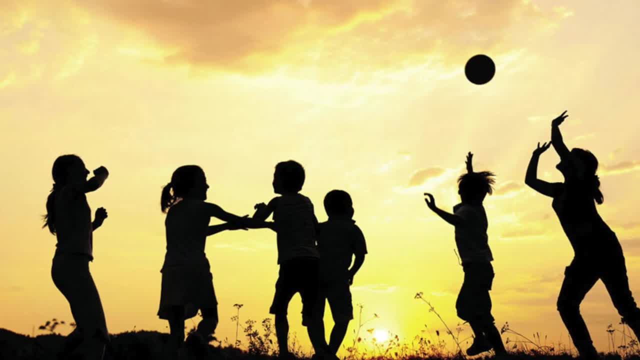 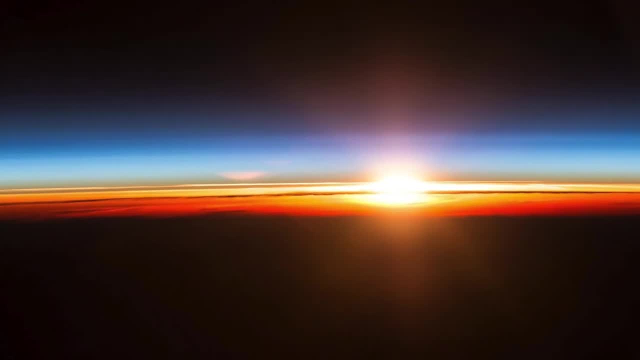 Think about the last time you spent a whole day outside in the yard playing, riding your bike or going to your favorite park. You start walking and playing as the sun rises over the horizon. You see the rays of the sun angle their way over the hills or through the 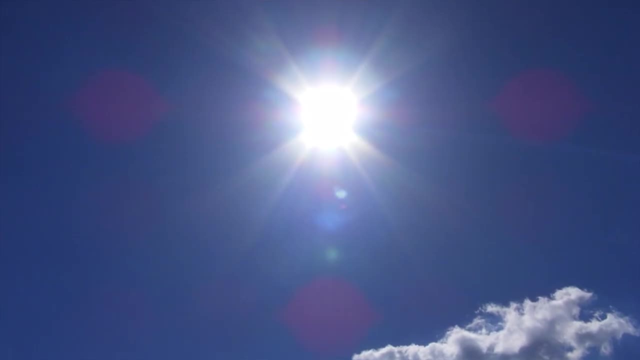 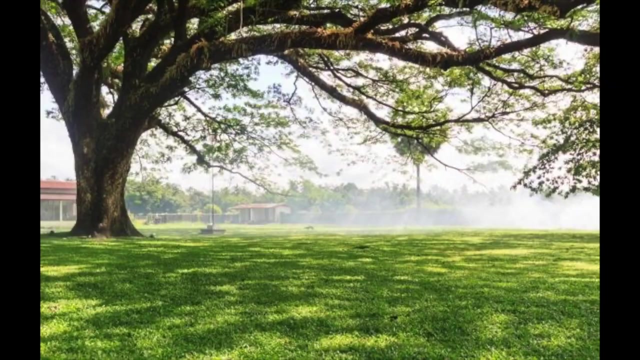 trees and feel slight warmth on your face. The sun moves steadily higher in the sky until at noon. it's beating nearly straight down on your sweaty face and is boiling hot Time to rest in the shade. Over six hours or so you experience the effect of changing light intensity on the ground as the 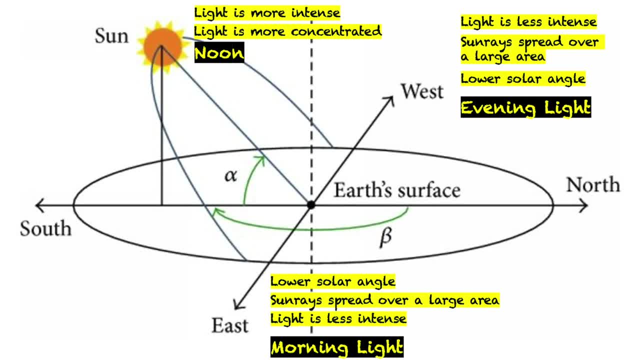 angle of the sun's rays changed. Early in the morning, Earth was illuminated by light that hit the surface at a very small angle. This is the time of the sun rising over the horizon. This is the time of the sun rising over the surface at a very small angle, perhaps only 10 degrees. The consequence: 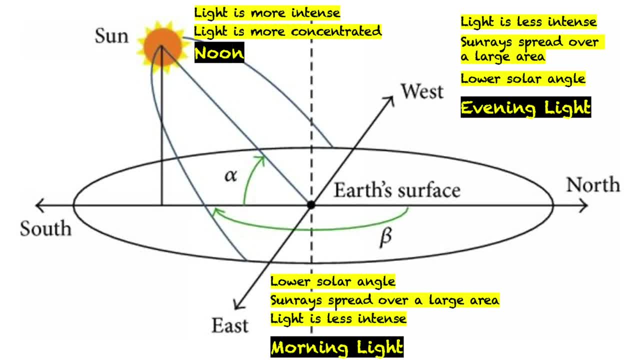 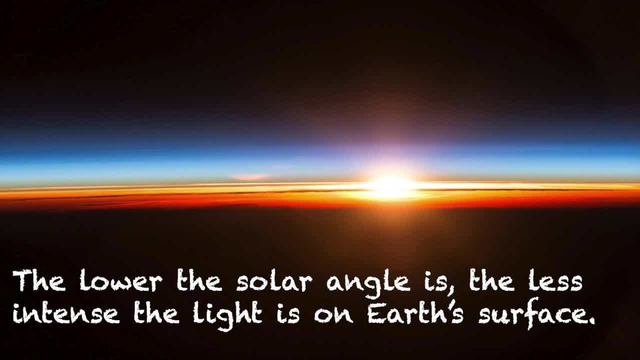 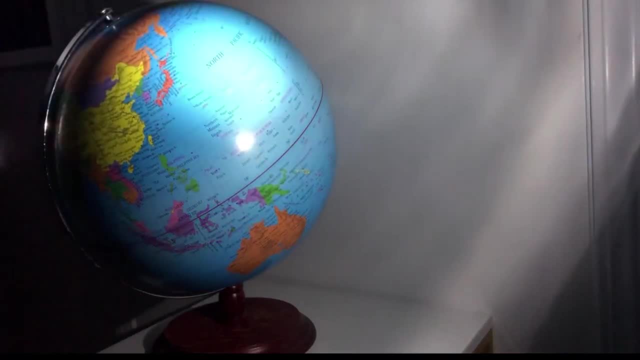 was that the beam was spread over a large area. The concentration of radiation was reduced because it was distributed across a large area. The lower the solar angle is, the less intense the light is on Earth's surface, because energy in the light beams spread over a larger area. You can observe: 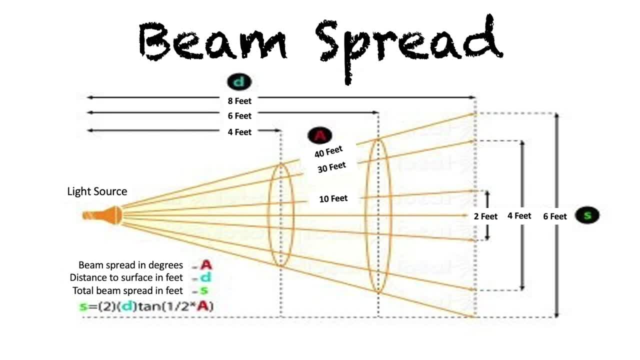 this effect when you shine a flashlight on the floor across the room. As compared to a shining light beam. the beam has exactly the same amount of light in both instances, but the beam at spot two spreads out over a larger area. The intensity of light per unit is less than. 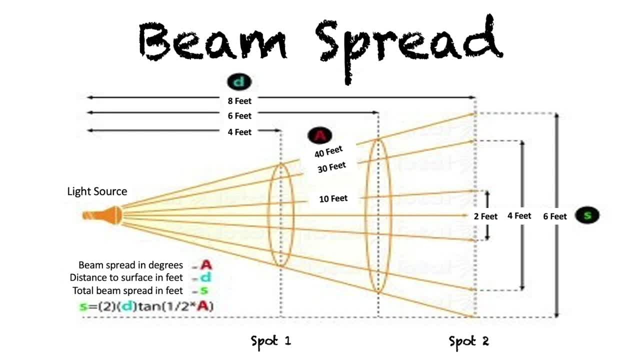 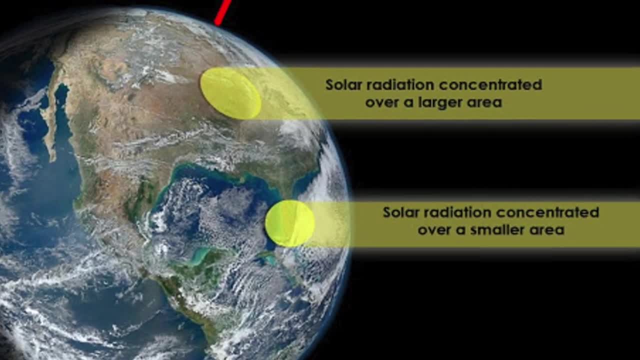 spot two than it is in spot one, which is illuminated from directly above 90 degrees Solar angle affects the intensity of light on an area, which in turn affects the amount of energy, which in turn affects the amount of heat transferred to an area of Earth during a